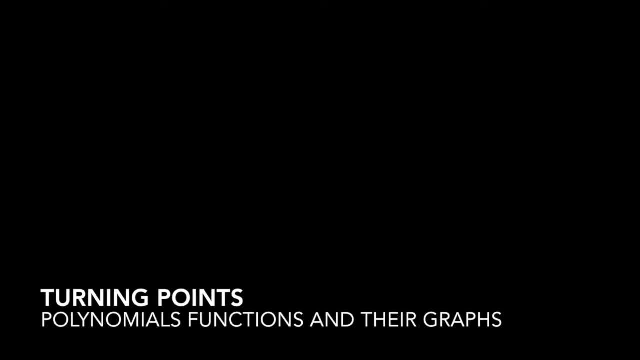 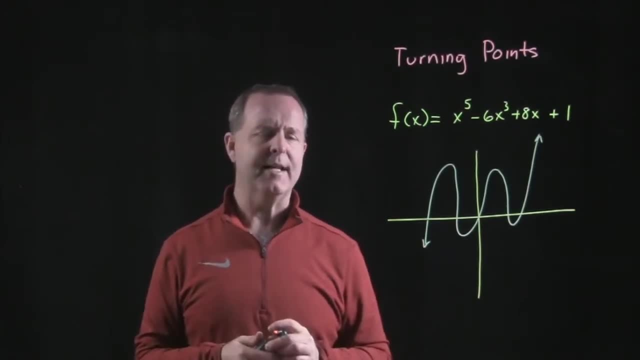 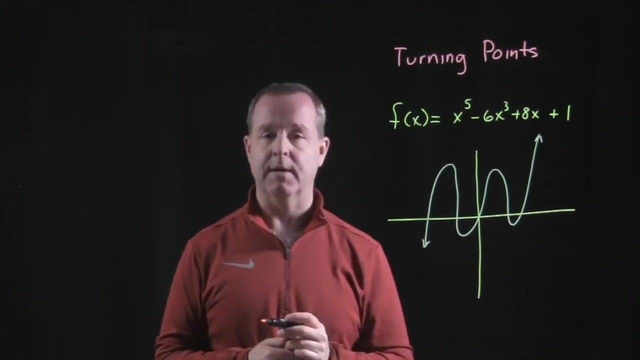 Maybe one last characteristic of polynomial functions that we can understand or have an idea about is this idea called turning points. Well, obviously, a turning point is where a graph turns around. This particular graph: if you were to graph it, go ahead and graph it now. if you want, x to the 5th minus x, cubed plus 8x plus 1.. This particular graph notice. 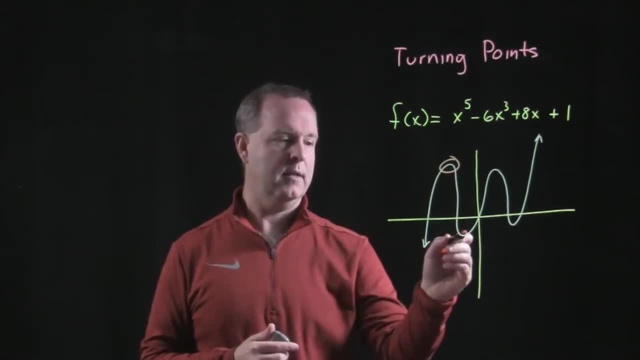 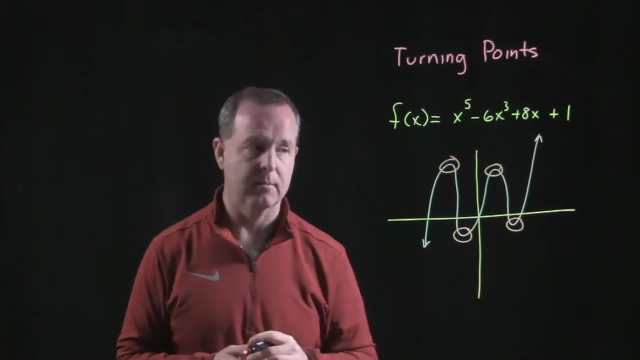 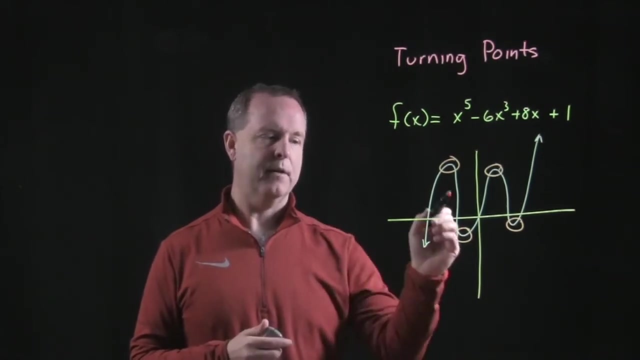 how many turning points it has: 1,, 2,, 3, and 4 turning points, And each turning point is a relative minimum or a maximum related to the rest of the graph. Well, what I'm curious about is how many turning points are there? There's 4.. That's not a coincidence. This. 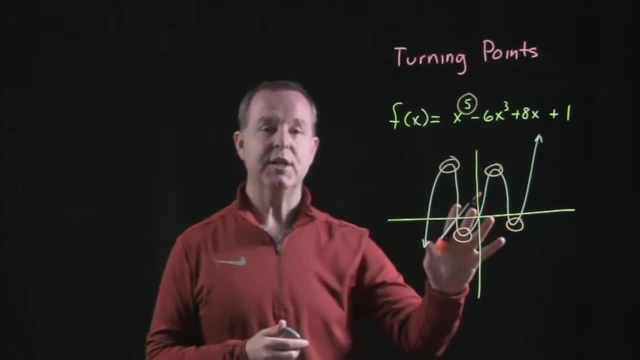 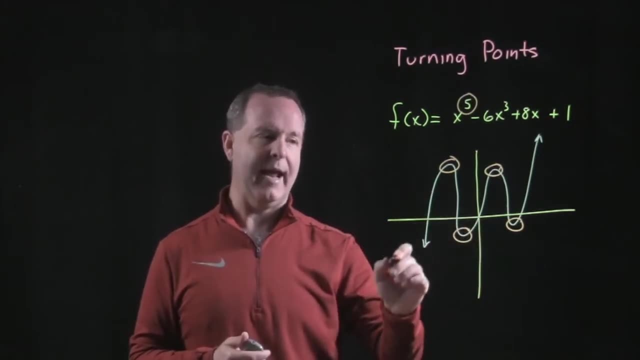 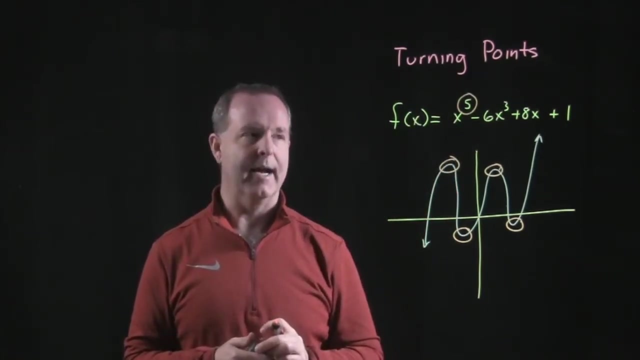 value right there, which is a 5,. the relationship between these two? well, let's say there is a relationship. At most, the number of turning points I'm going to have in a graph is always going to be one less than my leading coefficients or my highest index or the degree of my polynomial. 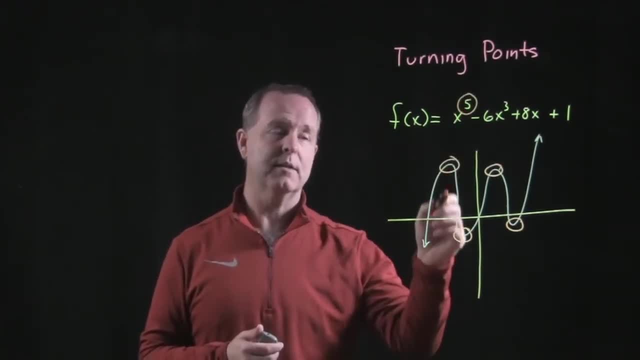 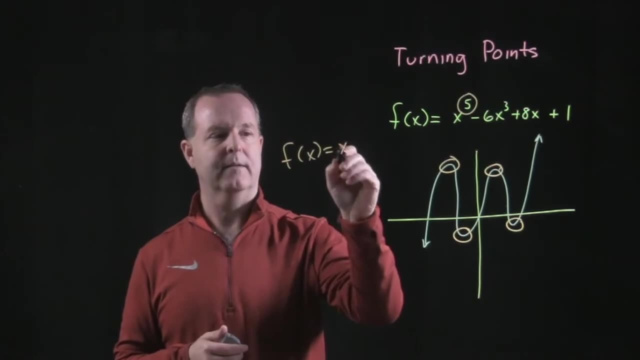 So if the degree of my polynomial is a 5, I'll have at most 4 turning points. If the degree of my polynomial, for example, is like x to the 7th, it has a 7th degree polynomial. so how many turning points are you going to expect? 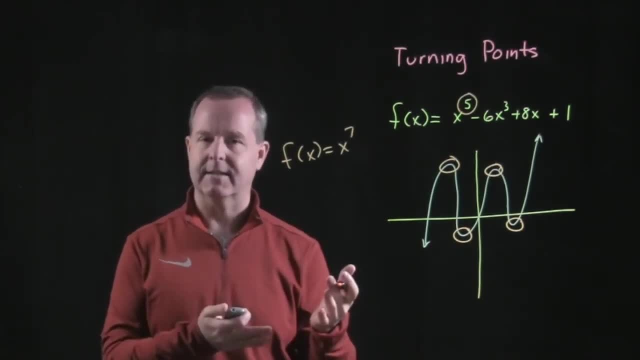 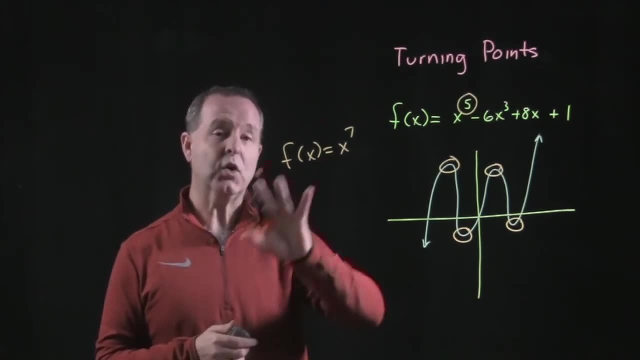 Well, at most there's going to be 6.. Not going to be 7,, not going to be 8,, not going to be 9, but at most there's going to be 6.. So turning points can help us continue to. 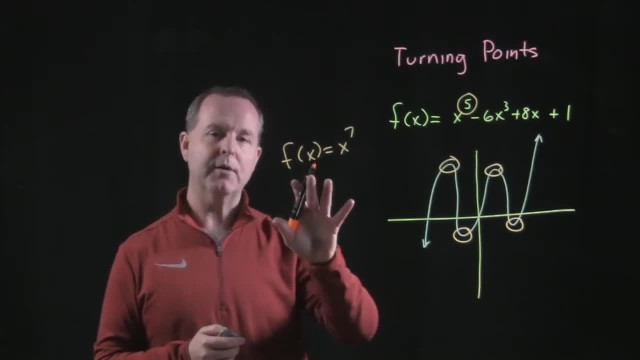 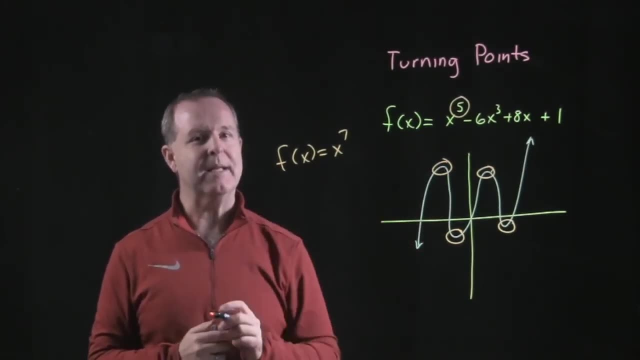 fill in some of the gaps, as we're learning how to model and graph a polynomial function And finding those particular turning points that are values of those. that's going to be a little bit more tricky And that's something that we're going to have to rely on our friends. 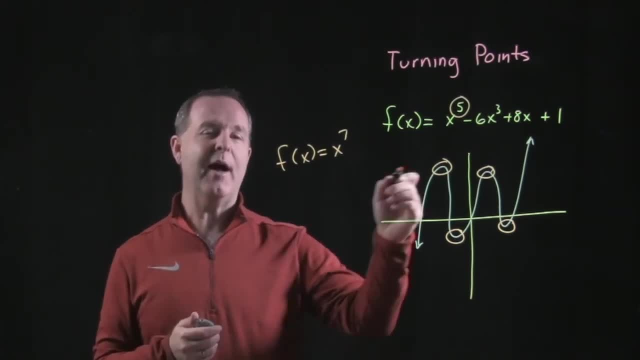 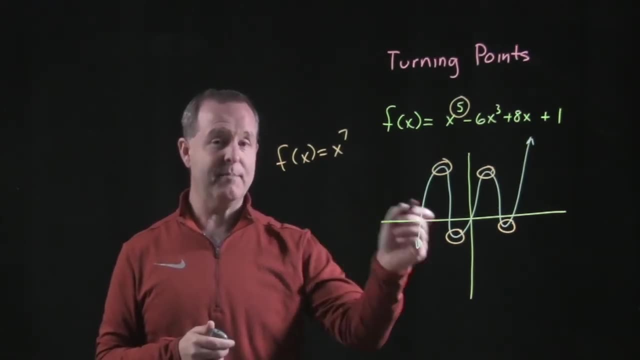 from calculus to help us out, But for us we know how many turning points there are, where they're exactly at, and identifying will be a little bit trickier. We'd always find maybe some test values and narrow it, but let's just let our friends in calculus deal with that part of it, alright.